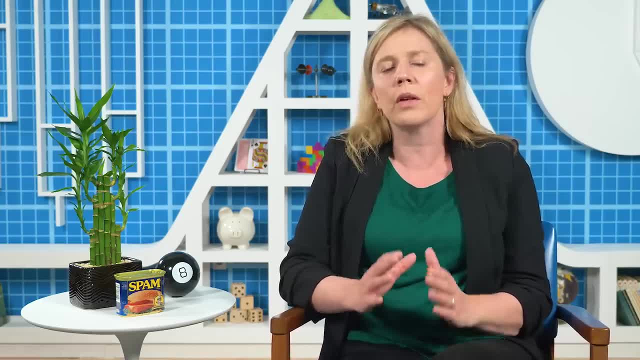 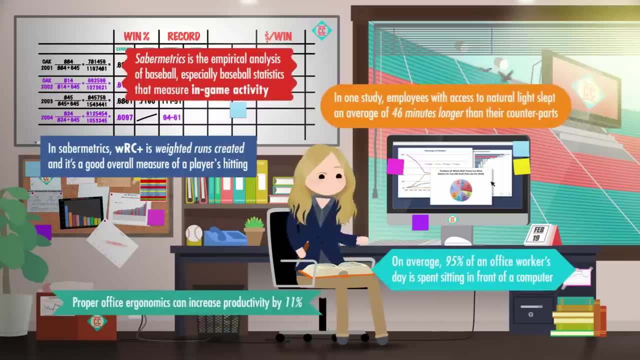 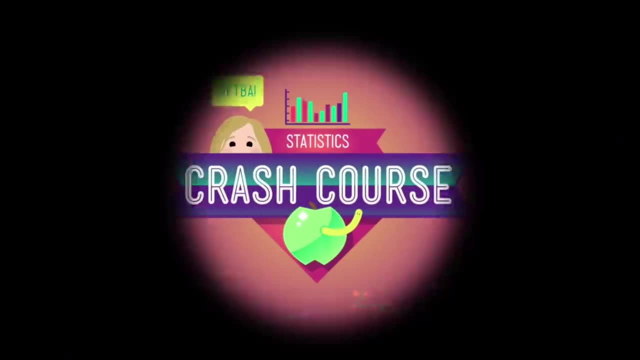 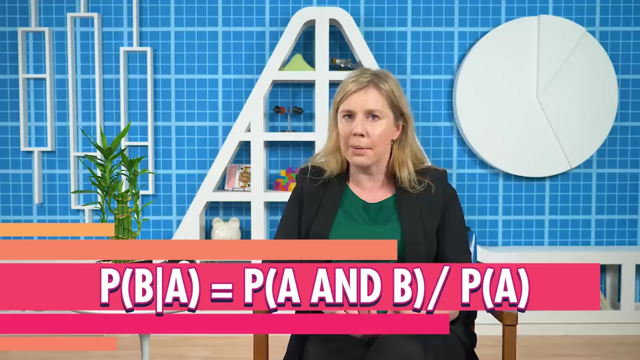 idea of why this is true and how this formula, with a few tiny tweaks, has really revolutionized the field of statistics. In general terms, conditional probability says that the probability of an event B, given that event A has already happened, is the probability of A and B happening together. 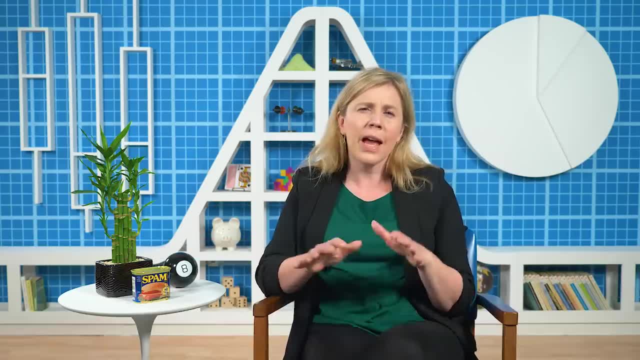 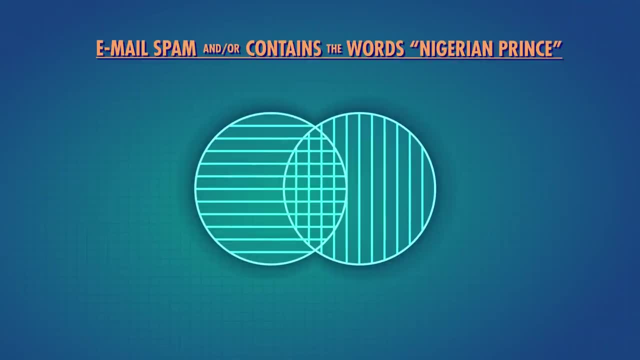 divided by the probability of A happening. That's the general formula, but let's look at a concrete example so we can visualize it. Here's a Venn diagram of two events: an email containing the words Nigerian Prince and an email being spam. So I get an email that has the words Nigerian Prince in it. 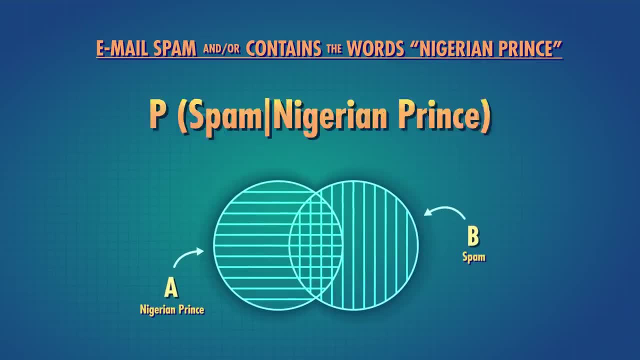 And I want to know what the probability is that this email is spam, given that I already know the email contains the words Nigerian Prince. This is the equation. Alright, let's take this apart a little. On the Venn diagram, I can represent the fact. 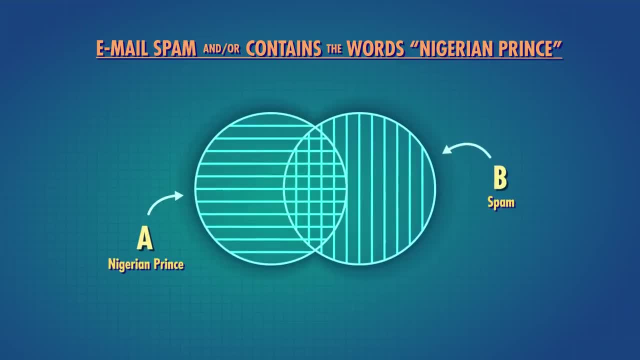 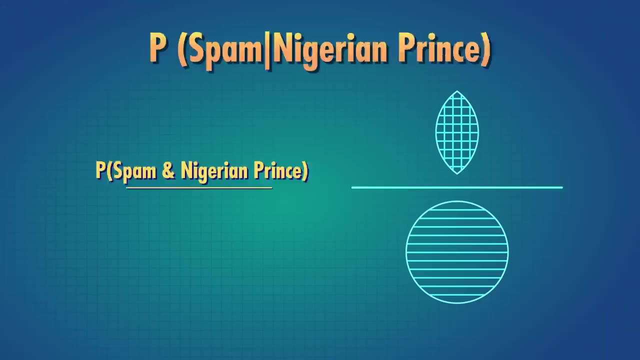 that I know the words Nigerian Prince already happened by only looking at the events where Nigerian Prince occurs. So just this circle. Now, inside this circle, I have two areas: Areas where the email is spam and areas where it's not. According to our formula, the probability of spam given Nigerian Prince is the probability. 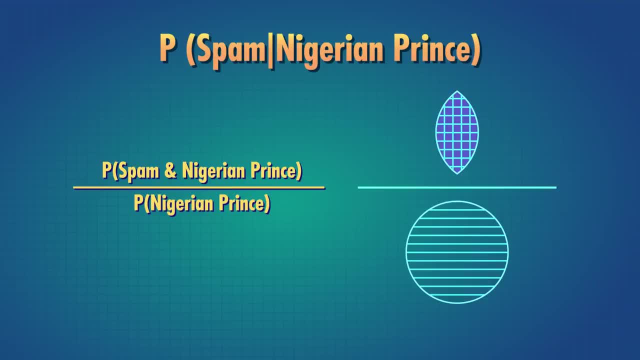 of spam and Nigerian Prince, which is this region where they overlap, divided by the probability of Nigerian Prince, which is the whole circle that we're looking at Now. if we want to know the proportion of times when an email is spam, we can look at this. 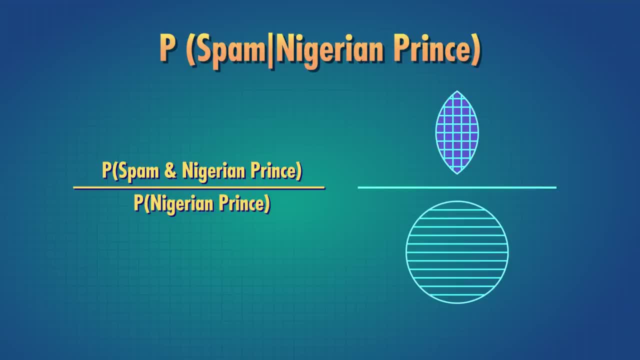 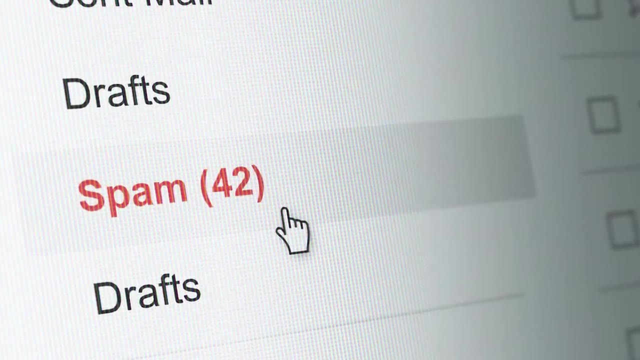 diagram, Given that we already know it has the words Nigerian Prince, we need to look at how much of the whole Nigerian Prince circle that the region with both spam and Nigerian Prince covers, And actually some email servers use a slightly more complex version of this example to filter. 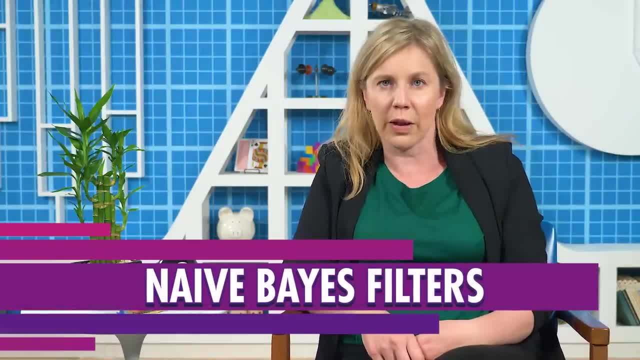 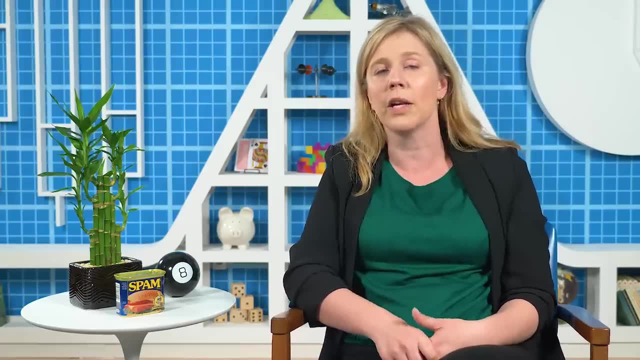 spam. These filters are called naive Bayes filters and thanks to them, you don't have to worry about seeing the desperate pleas of a surprisingly large number of Nigerian Prince messages. The Bayes in naive Bayes comes from the Reverend Thomas Bayes, a Presbyterian minister who broke 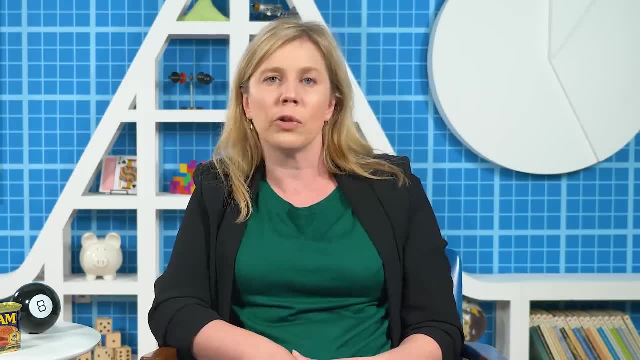 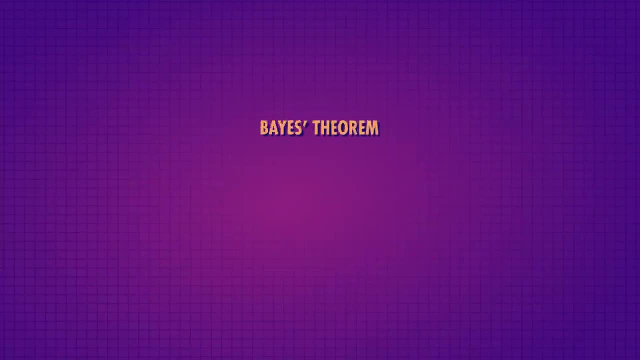 up his days of prayer with math. His largest contribution to the field of math and statistics is a slightly expanded version of our conditional probability formula. Bayes' theorem states that the probability of B given A is equal to the probability of A given B times the 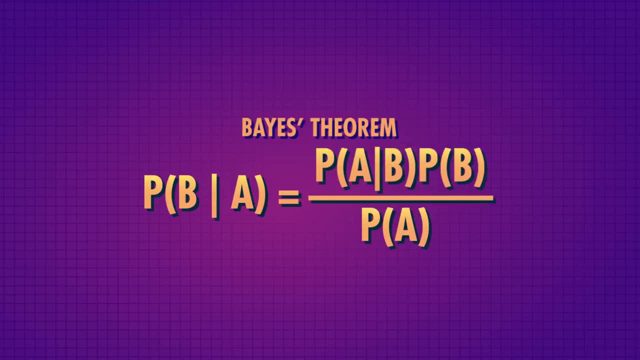 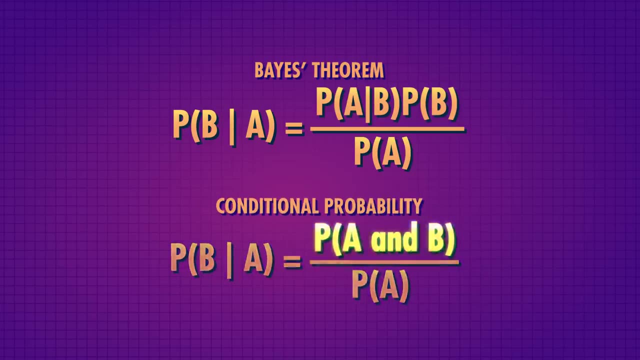 probability of B all divided by the probability of A. You can see this is just one step away from our conditional probability. It's just the same as our conditional probability formula. probability formula: The only changes in the numerator where probability A and B. 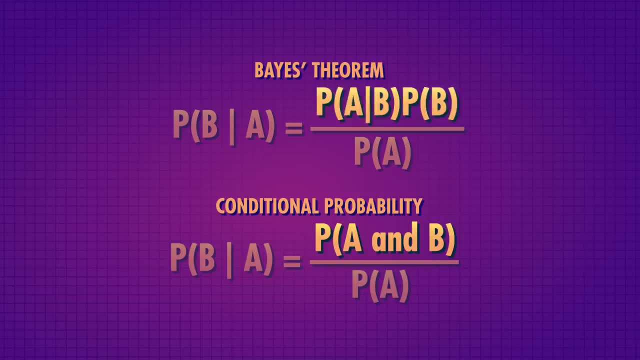 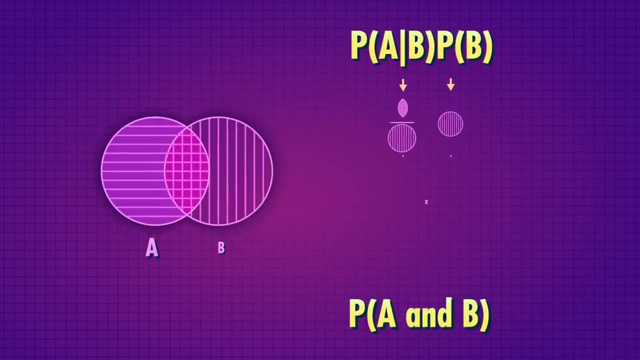 is replaced with probability A, given B times probability B. While the math of this equality is more than we're gonna go into here, you can see with some Venn diagram algebra why this is the case. In this form, the equation is known as Bayes. 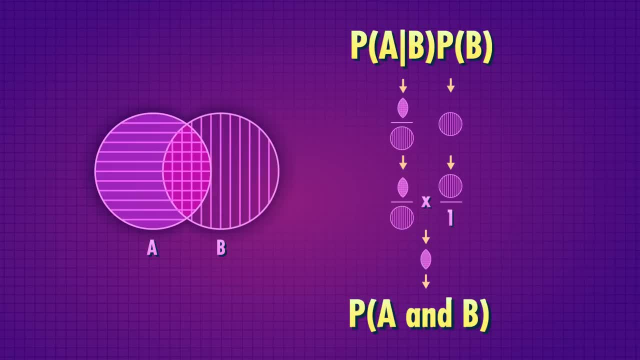 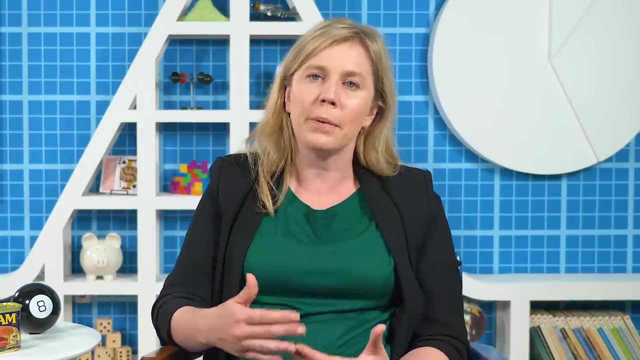 theorem, and it's inspired a strong movement in both the statistics and science worlds. Just like with your emails, Bayes theorem allows us to figure out the probability that you have a piece of spam on your hands using information that we already have: the presence of the words Nigerian Prince We. 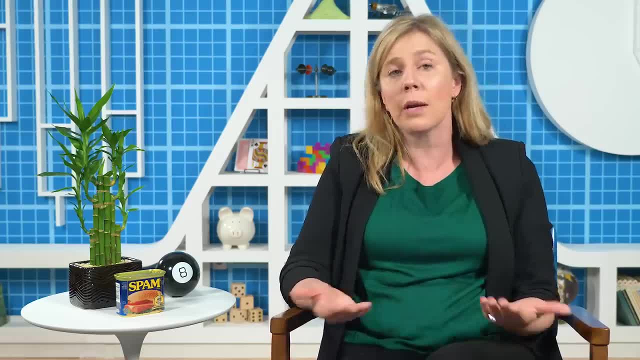 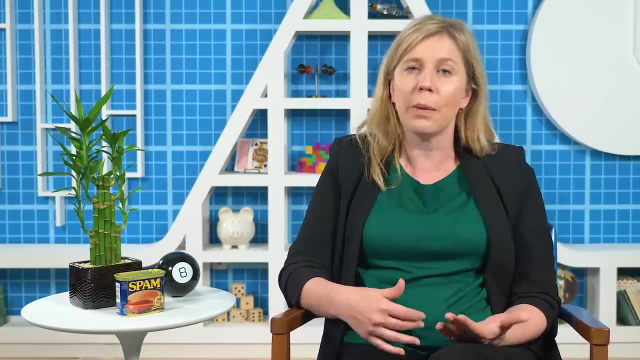 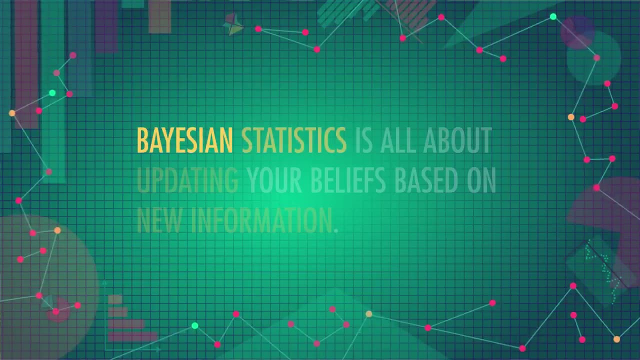 can also compare that probability to the probability that you just got a perfectly valid email about Nigerian Prince's. If you just tried to guess your odds of an email being spam based on the rate of spam to non-spam email, you'd be missing some pretty useful information. the actual words in the email: Bayesian. 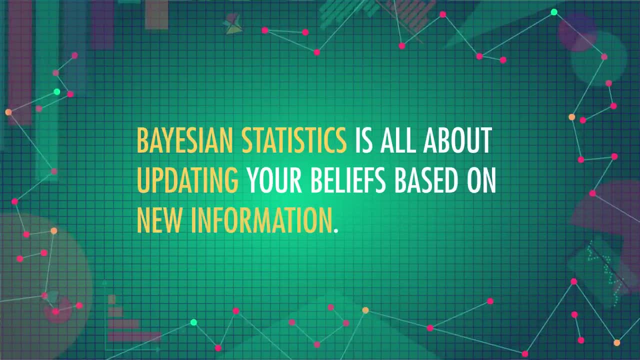 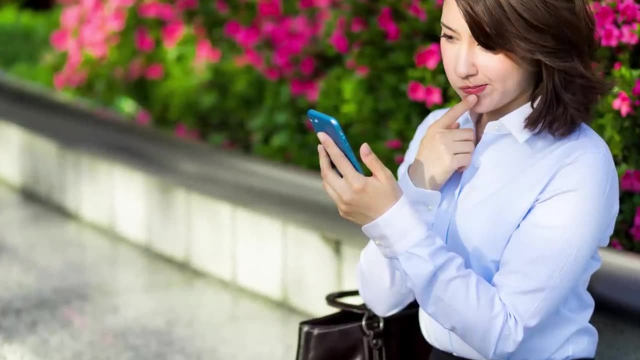 statistics is all about updating your beliefs based on new information. When you receive an email, you don't necessarily think it's spam, but once you see the word Nigerian, you're suspicious. It may just be your Aunt Judy telling you what she saw on the news, but as soon as you see Nigerian and Prince, 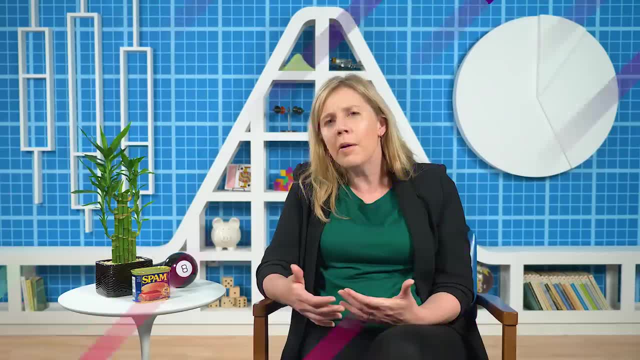 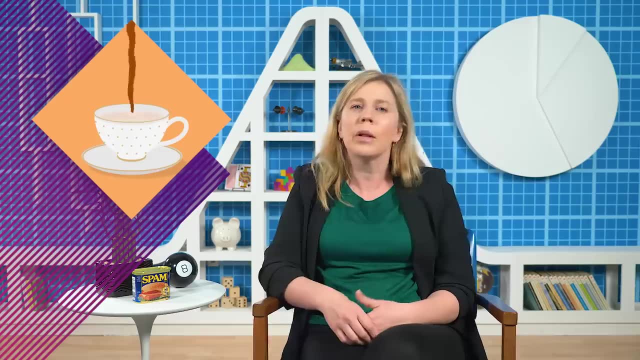 together, you're pretty convinced this is junk mail. Remember our lady tasting tea example, where a woman claimed to have superior taste buds that allowed her to know with one sip whether tea or milk was poured into a cup first. When you're watching this lady predict whether the tea or milk was poured first each. 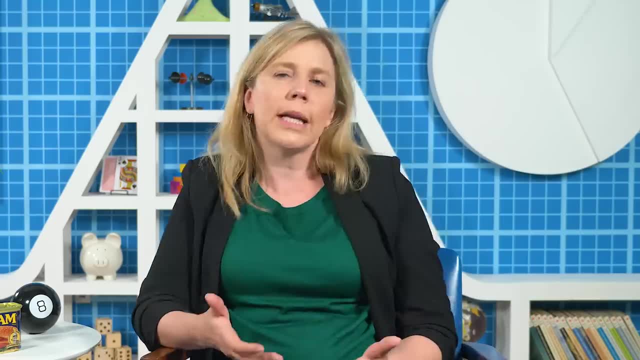 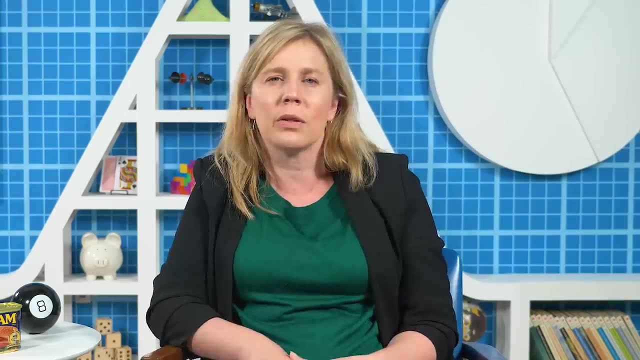 correct guess makes you believe her just a little bit more. A few correct guesses may not convince you, but each correct prediction is a little more evidence. she has some weird super tasting tea powers. Reverend Bayes described this idea of updating in a thought experiment. Say that you're standing next to a pool. 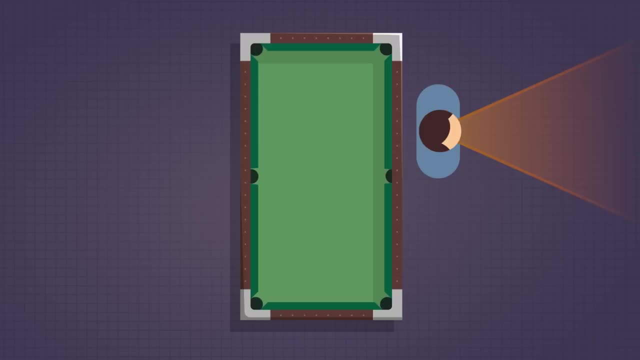 table, but you're faced away from it so you can't see anything on it. You then have your friend randomly drop a ball into the table- and this is a special, very even table- so the ball has an equal chance of landing anywhere on it You're. 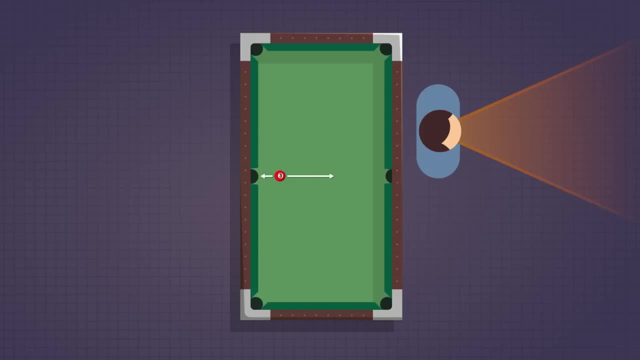 then therefore placed here inside the pool. Your mission is to guess how far to the right or left this ball is. You have your friend drop another ball onto the table and report whether it's to the left or to the right of the original ball, The 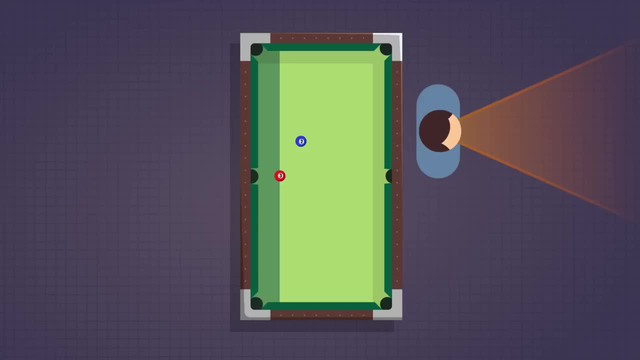 new ball is to the right of the original, so we can update our belief about where the ball is. If the original is more towards the left, then most of the new balls will fall to the right of the original ball, just because there's more. 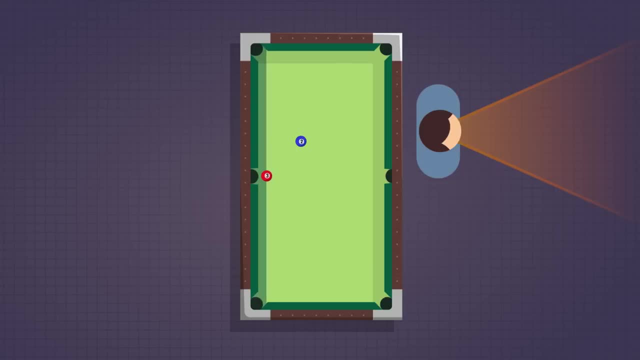 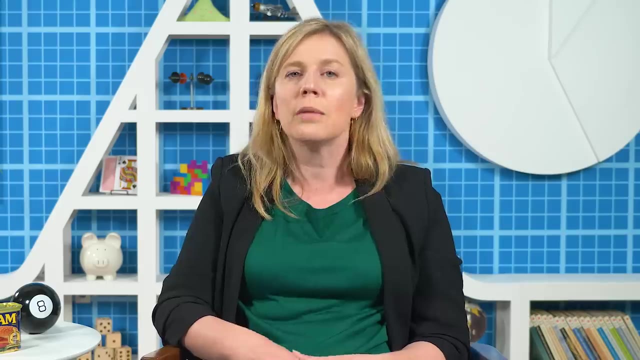 area there And the further to the left the original ball is, the higher the ratio of new rights to lefts ball is to the right of the original ball. that means there's a better chance that our original is more to the left side of the table than the right, since there would be 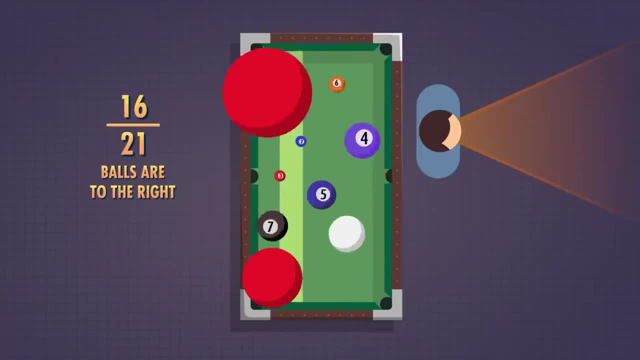 more room for the new ball to land. Each ball that lands to the right of the original is more evidence that our original is towards the left of the table. But if we get a ball landing on the left of our original, then we know the original ball. 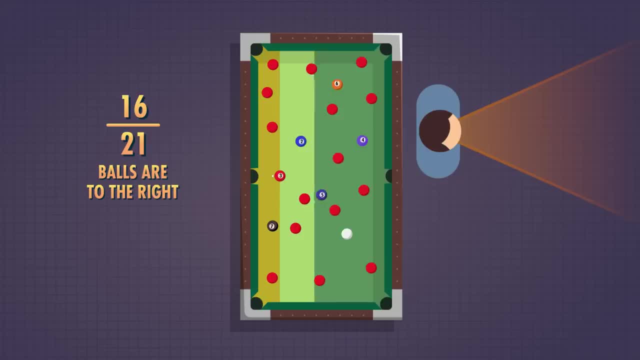 is not at the very left edge of the table. Again, each new piece of information allows us to change our beliefs about the location of the ball, And changing beliefs is what Bayesian statistics is all about. Outside thought experiments, Bayesian statistics is being used in many different ways from 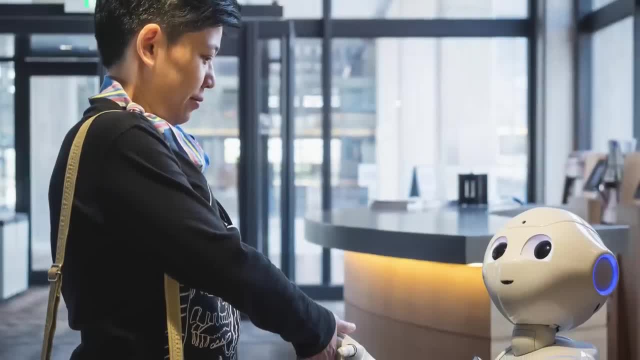 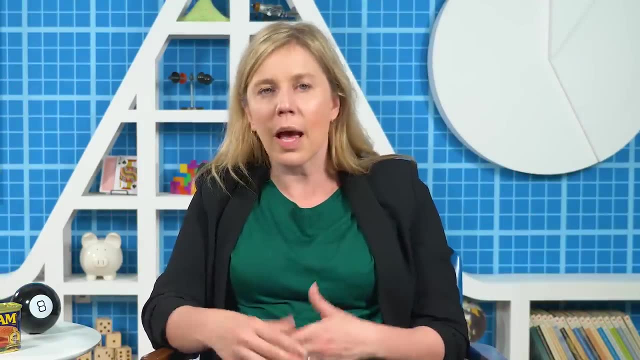 comparing treatments in medical trials to helping robots learn language. It's being used by cancer researchers, ecologists and physicists, And this method of thinking about statistics- updating existing information with what's come before- may be different from the logic of some of the statistical tests that you've. 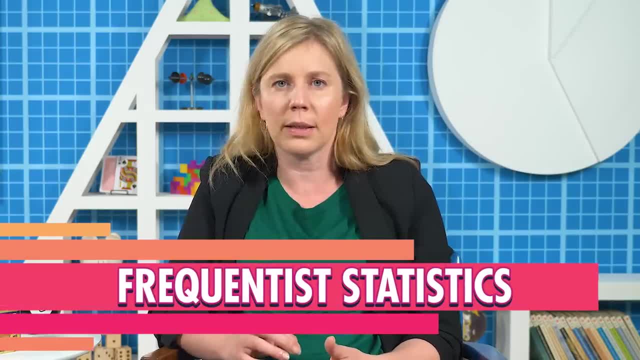 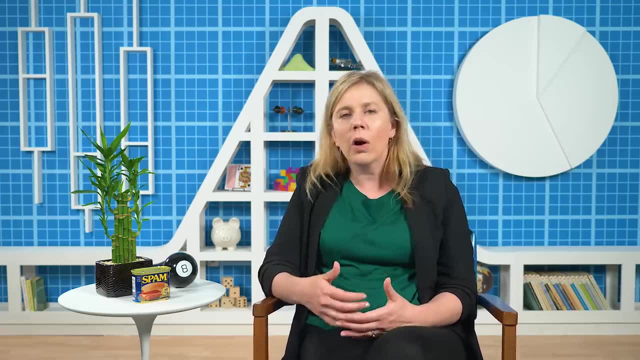 heard of. like the t-test, Those frequentist statistics can sometimes be more like probability done in a vacuum, less reliant on prior knowledge, And when the math of probability gets hard to wrap our heads around, we can use simulations to help see these rules in action. 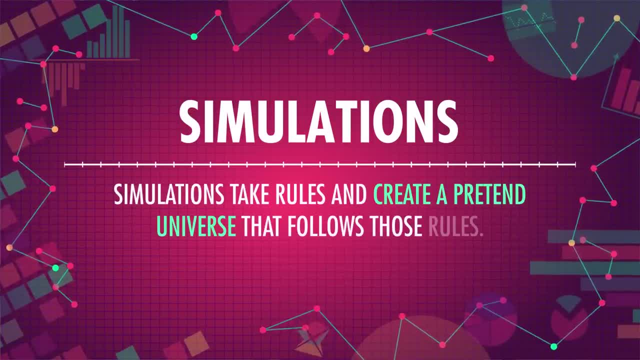 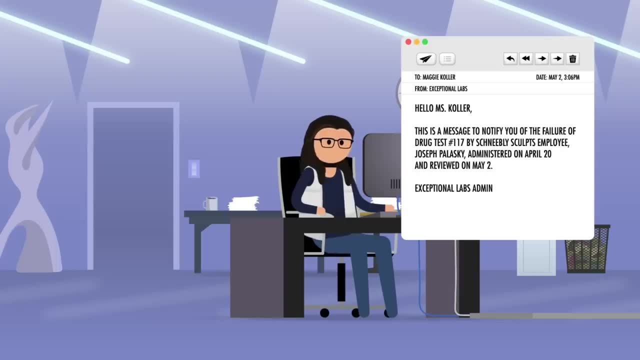 Simulations, take rules and create a pretend universe that follows those rules. Let's say you're the boss of a company and you receive news that one of your best employees, Joe, has failed a drug test. It's hard to believe And you remember seeing this thing on YouTube that told you how to figure out the probability. 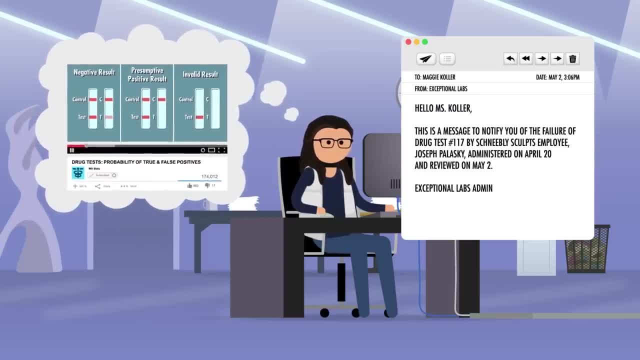 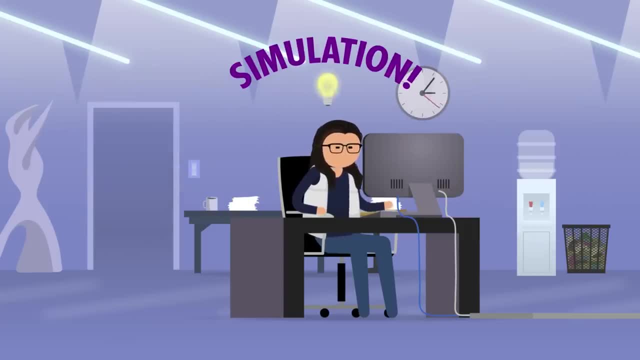 that Joe really is on drugs, Given that he got a positive test. You can't remember exactly what the formula is, but you can always run a simulation. Simulations are nice because we can just tell our computer some rules and it will randomly. 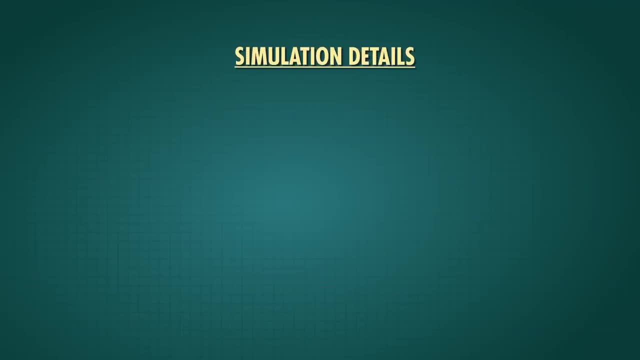 generate data based on those rules. For example, we can tell it the base rate of people in our state that are on drugs, the sensitivity of the drug test and the specificity of the test. Then we ask our computer to generate 10,000 simulated people and tell us what percent. 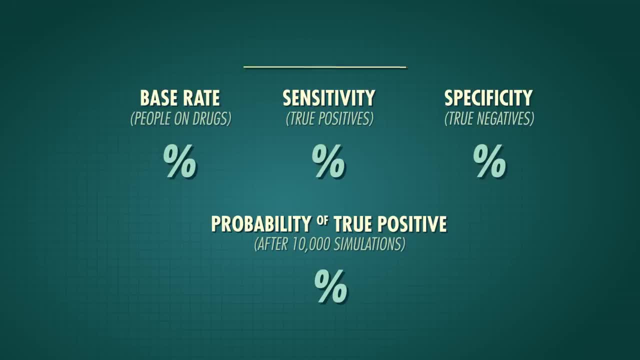 of the time, the people with positive drug tests were actually on drugs, If the drug Joe tested positive for, in this case, Glitter Stim, is only used by about 5% of the population and the test for Glitter Stim has a 90% sensitivity and a 95% specificity. 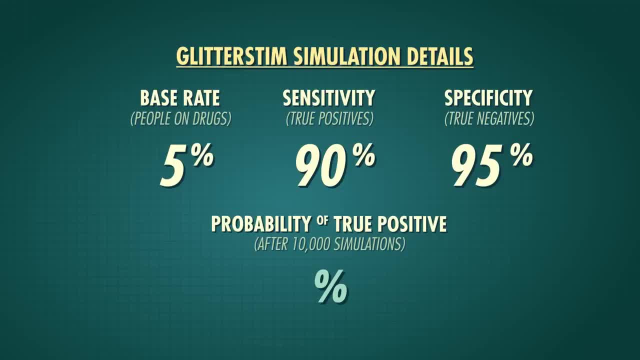 I can plug that in and ask the computer to simulate 10,000 people according to these rules, And when we ran the simulation, only 49.2% of the people who tested positive were actually using Glitter Stim. So I should probably give Joe another chance or another test. 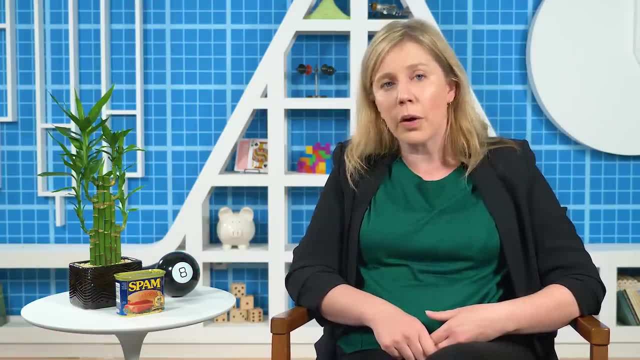 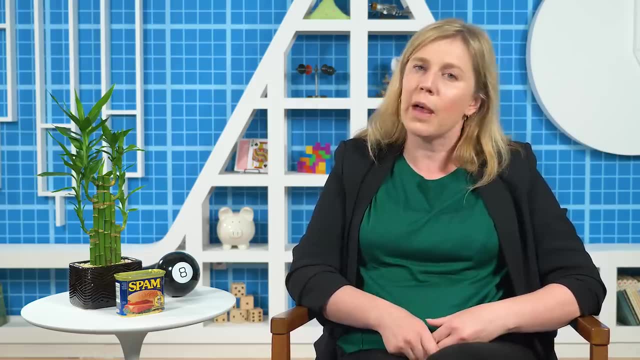 And if I did the math, I'd see that 49.2% is pretty close, since the theoretical answer is around 48.6%. Simulations can help reveal truths about probability even without formulas. They're a great way to demonstrate probability and create intuition that can stand alone. 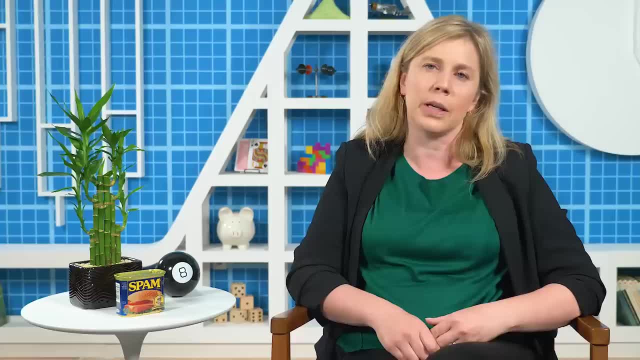 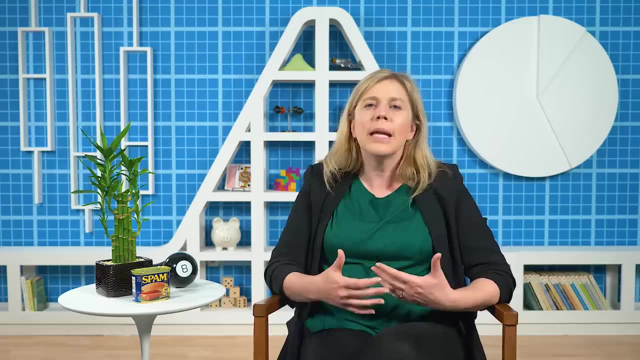 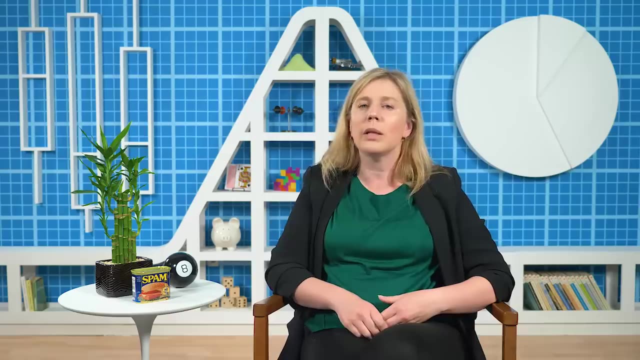 or build on top of more mathematical approaches to probability. Let's use a simulation to demonstrate an important concept in probability that makes it possible to use samples of data. In fact, we were secretly relying on it when we used empirical probabilities- like how many times I got tails when flipping a coin 10 times- to estimate theoretical probabilities. 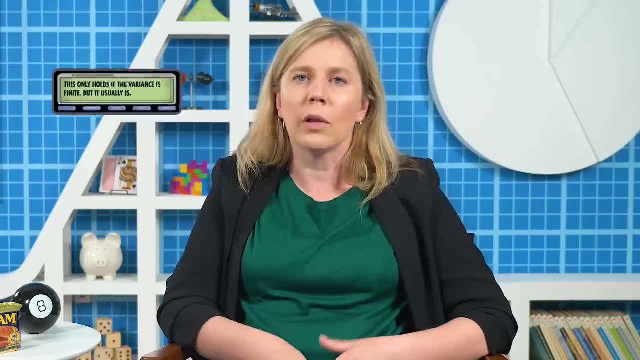 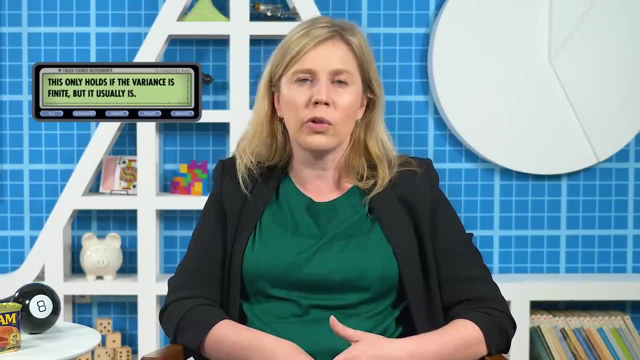 like the true probability of getting tails In its weak form, law of large numbers tells us that as our samples of data get bigger and bigger and bigger our sample mean will be arbitrarily close to the true population mean. Let's see a simulation. 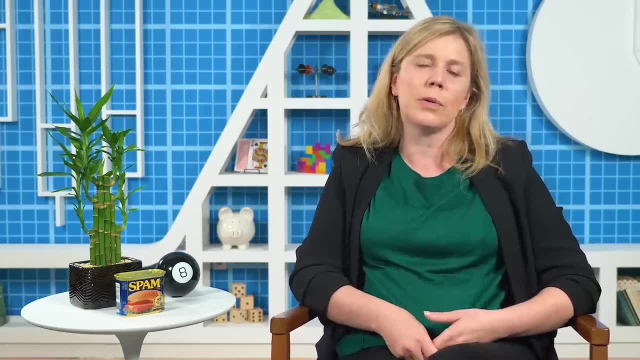 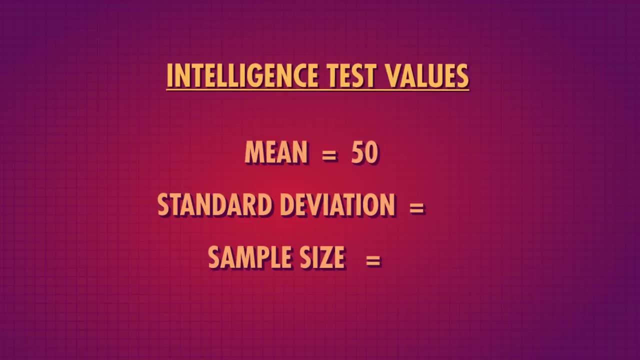 And if you want to follow along or run it on your own, instructions are in the description below. In this simulation we're picking values from a new intelligence test, from the normal distribution that has a mean of 50 and a standard deviation of 20.. 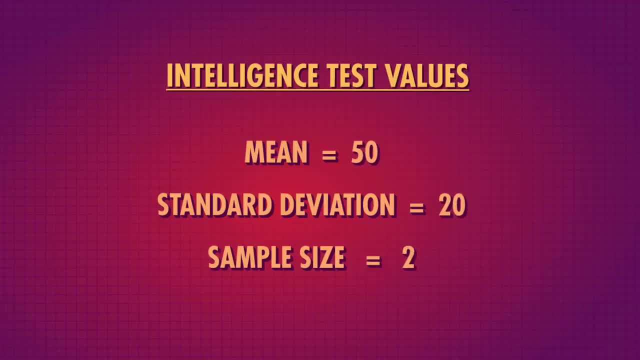 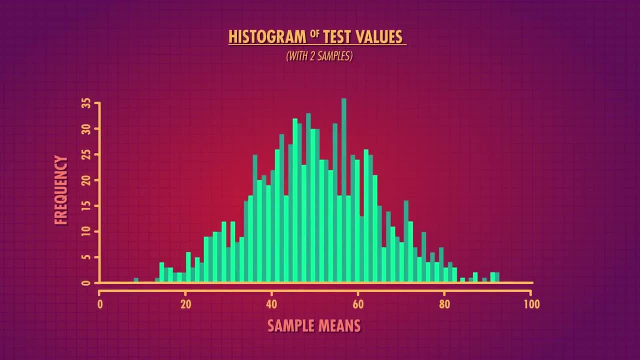 When you have a very small sample size, say 2,, your sample means are all over the place. You can see that pretty much anything goes. We get means between 5 and 95. And this makes sense. When we only have two data points in our sample, it's not that unlikely that we'll get two. 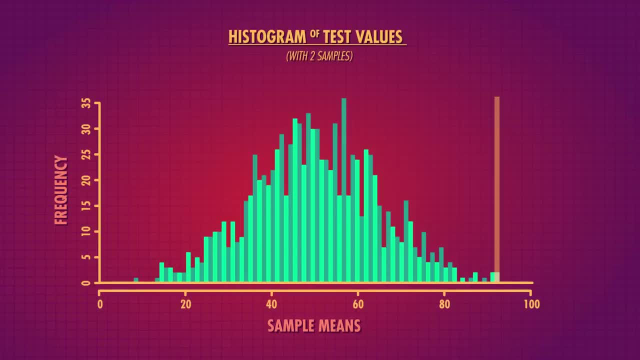 really small numbers or two pretty big numbers, which is why we see both low and high sample means, Though we can tell that a lot of the means are around the true mean of 50, because the histogram is the tallest at values around 50.. 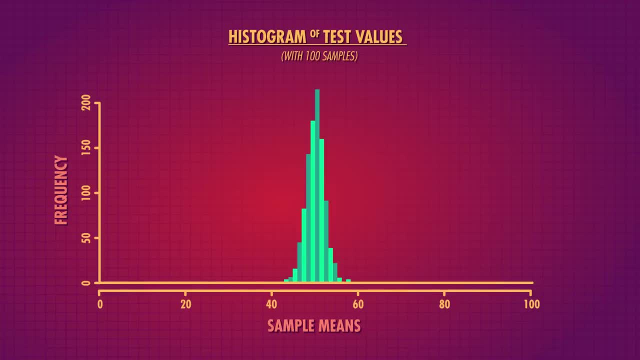 But once we increase the sample size, even to just 100 values, you can see that the sample means are mostly around the real mean of 50. In fact, all of the sample means are within 10 units of the true population mean, And when we go up to 1,000, just about every sample means are within 10 units of the true 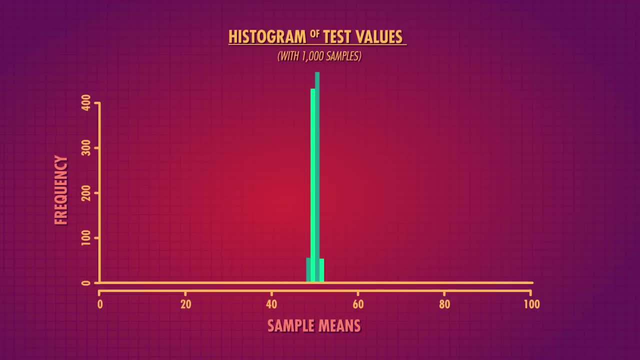 population mean. And when we go up to 1,000, just about every sample means are within 10 units of the true population mean. And when we go up to 1,000, just about every sample means are within 10 units of the true. 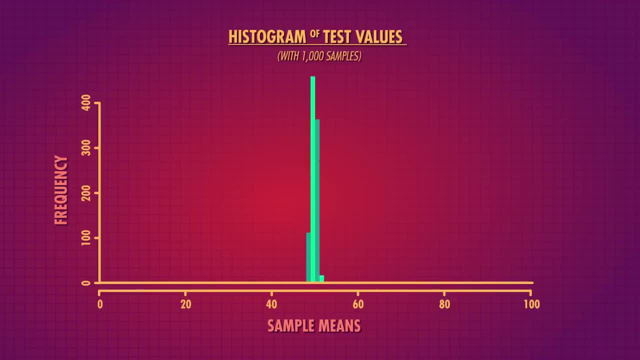 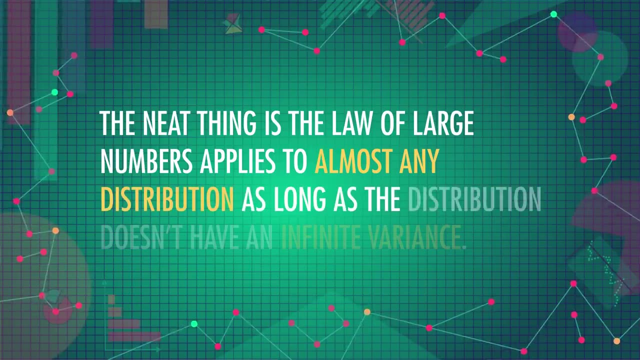 population mean. And when we run this simulation over and over and over and over, you'll see pretty similar results. The neat thing is the law of large numbers applies to almost any distribution, as long as the distribution doesn't have an infinite variance. 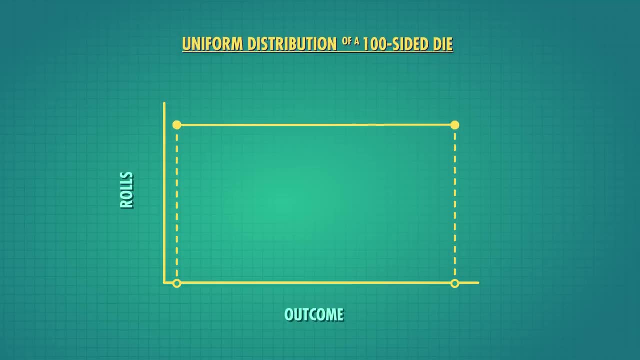 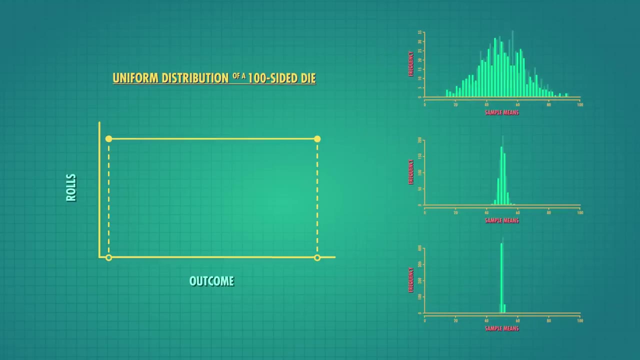 Take the uniform distribution, which looks like a rectangle. Imagine a 100-sided die. Every single value is equally probable. Even the sample means that are selected from a uniform distribution get closer and closer to the true mean of 50. So if we run this simulation over and over and over, we'll see pretty similar results. The law of large numbers is the evidence we need to feel confident that the mean of the samples we analyze is a pretty good guess for the true population mean, And the bigger our samples are, the better we think the guess is. This property allows us to make guesses about populations based on samples. 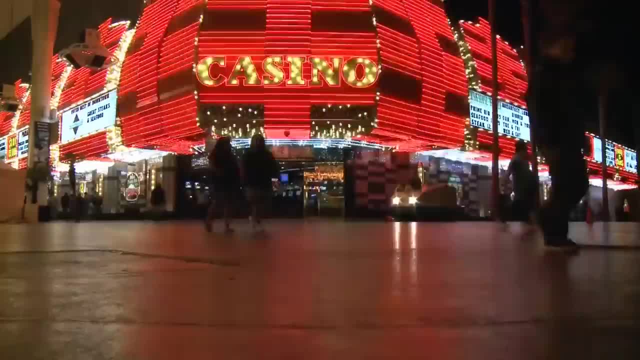 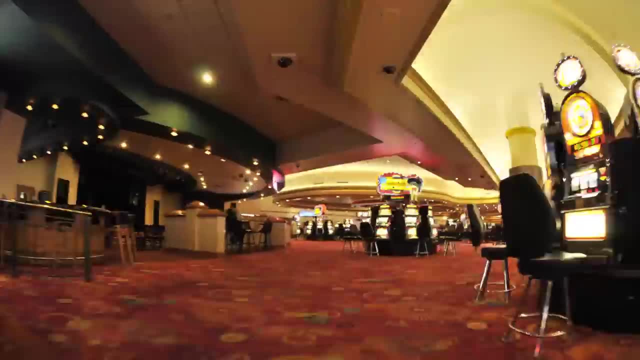 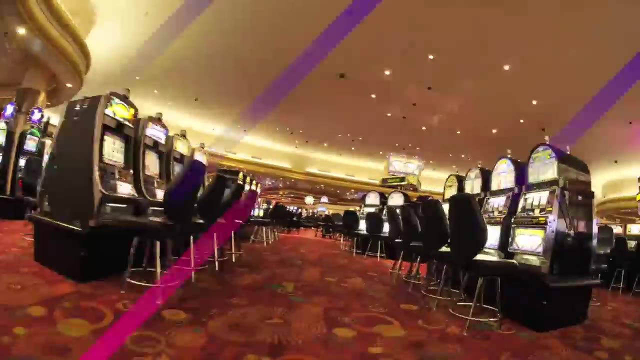 It also explains why casinos make money in the long run over hundreds of thousands of payouts and losses, even if the experience of each person varies a lot. The casino looks at a huge sample, every single bet and payout, whereas your sample as a individual is smaller and therefore less likely to be representative. 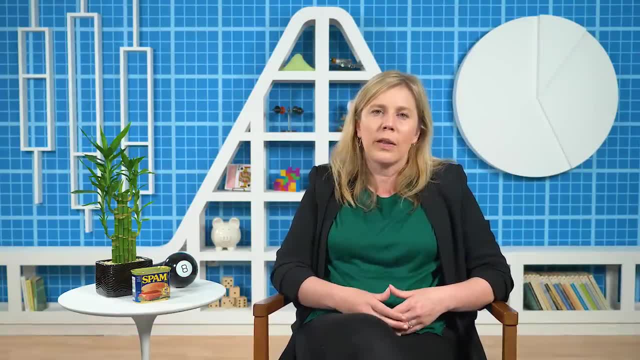 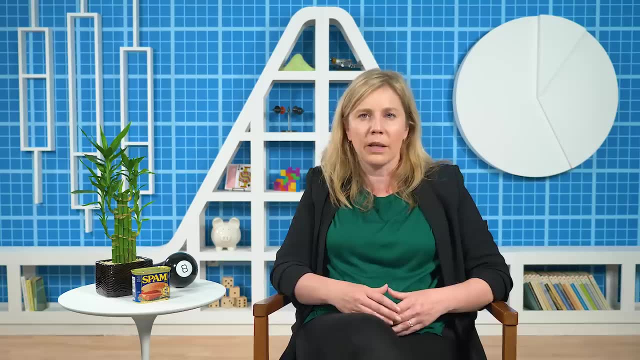 Each of these concepts can help us another way, Another way to look at the data around us. The Bayesian framework shows us that every event or data point can and should update your beliefs, but it doesn't mean you need to completely change your mind. 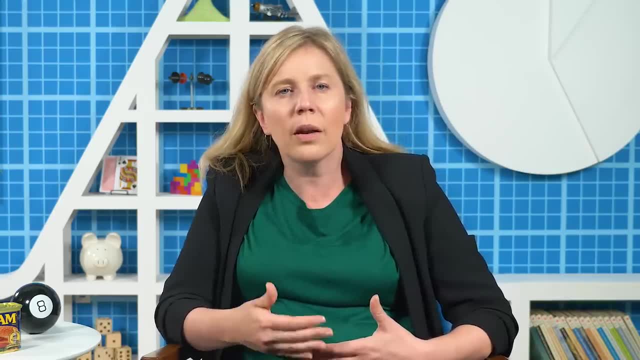 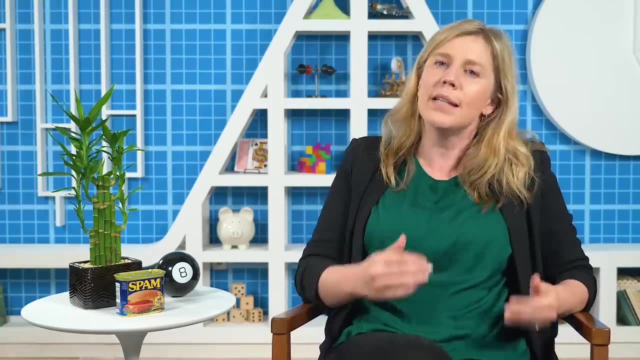 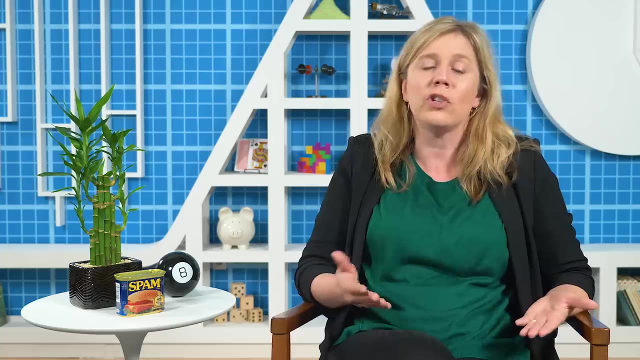 And simulations allow us to build upon these observations when the underlying mechanics aren't so clear. We're continuously accumulating evidence and modifying our beliefs every day, adding today's events to our conceptions. And hey, maybe one day we'll all sincerely start emailing each other about Nigerian. 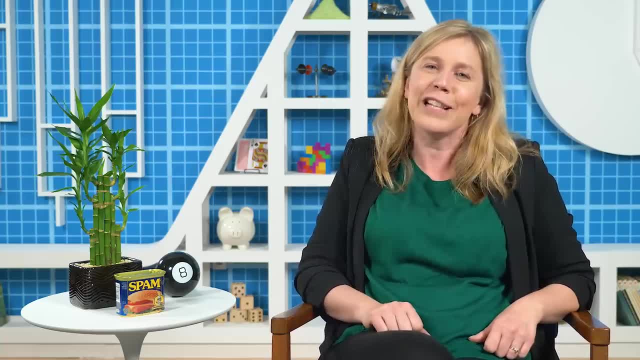 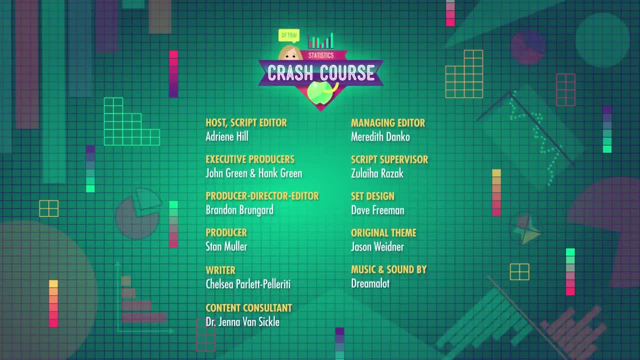 princes, and then we're going to have to do some belief updating. Thanks for watching. I'll see you next time. Crash Course Statistics is filmed in the Chad and Stacey Emigholtz Studio in Indianapolis, Indiana, And it's made with the help of all these nice people. 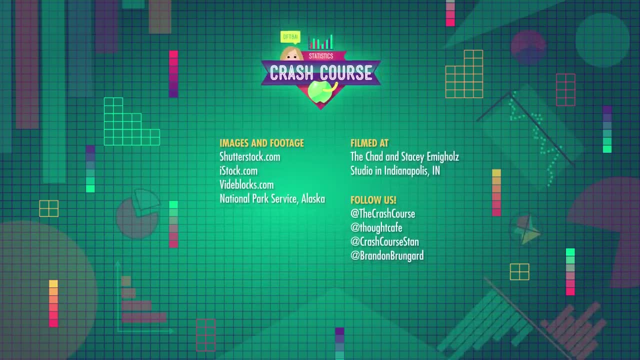 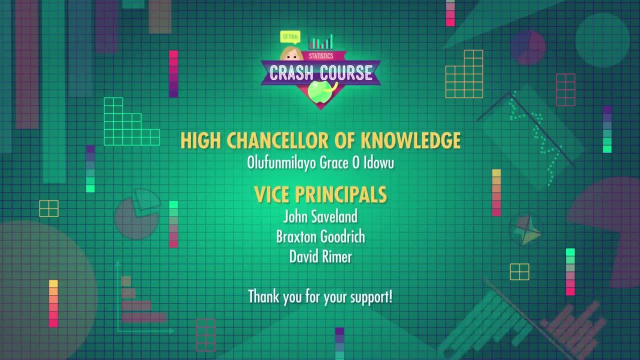 Our animation team is Thought Cafe. If you'd like to keep Crash Course free for everyone forever, you can support the series at Patreon, a crowdfunding platform that allows you to support the content you love, And thank you to all our patrons for your continued support. 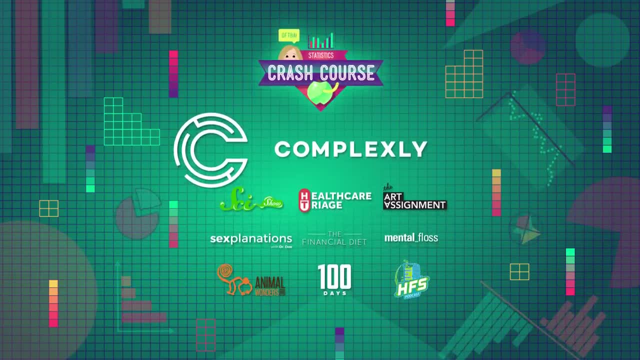 Crash Course is a production of Complexly. If you like content designed to get you thinking, check out some of our other channels at Complexlycom. Thanks for watching. 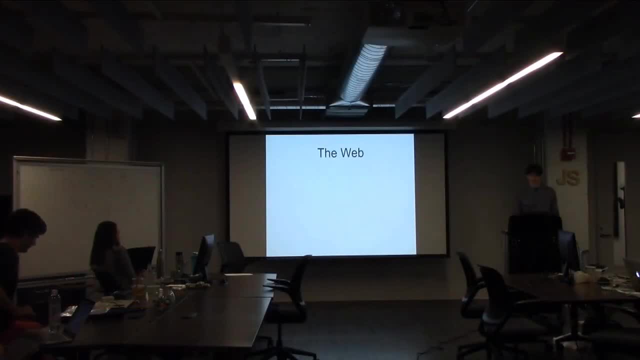 My name is James Bird and I'm here to talk about web accessibility. So you can think of the web a lot like you can think of a public library: It's a giant store of information available to everyone that people from all over can go to. 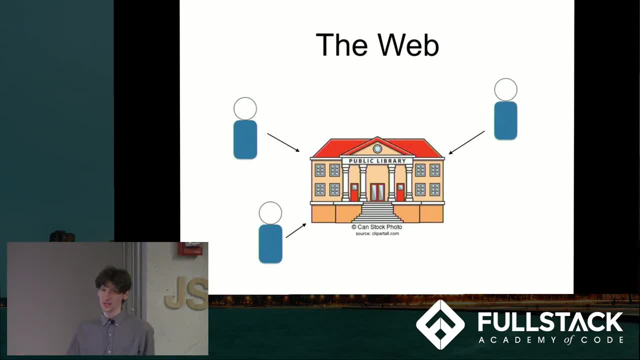 However, do you see a problem in this image? If you can't get upstairs, you're probably going to have a little bit of trouble getting into the library, Unless you have an on-access ramp. Web accessibility is basically building access ramps to the web. 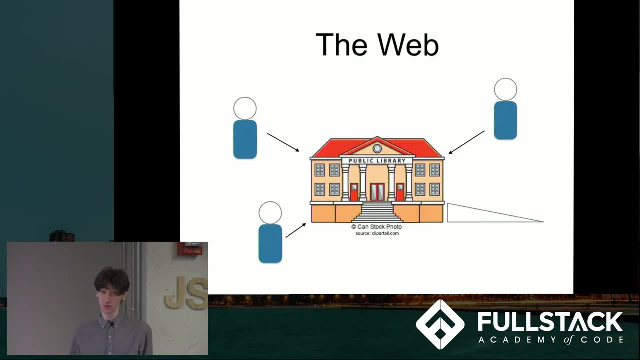 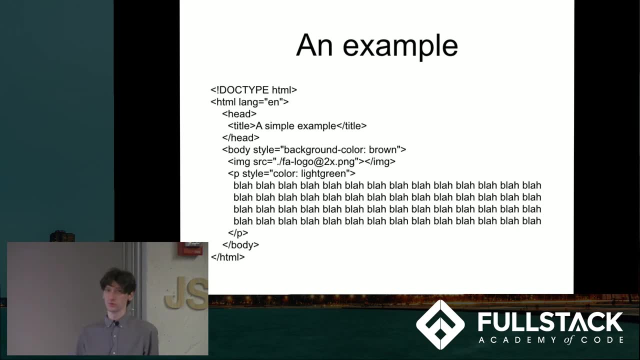 and making sure that everyone can access everything in the web equally and on the same level. So here's an example. This code more or less looks fine. It's not great code, It's kind of a crappy website probably, But nonetheless it works. 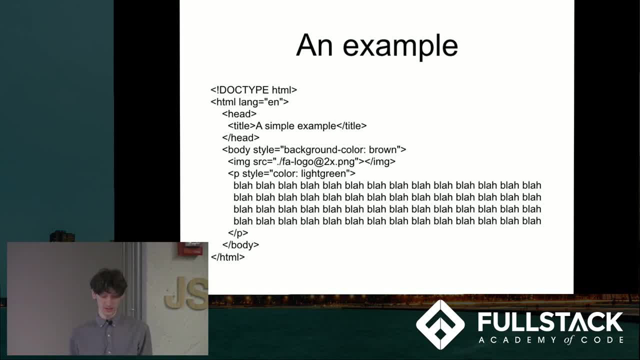 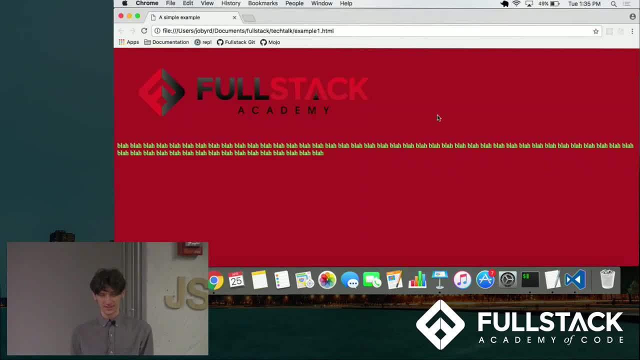 However, there are some problems that are not immediately apparent from just looking at the code. So here I'm going to open up the web page and we'll see the problem. See, not only is this ugly, there's also the fact that if you have red-green color blindness, 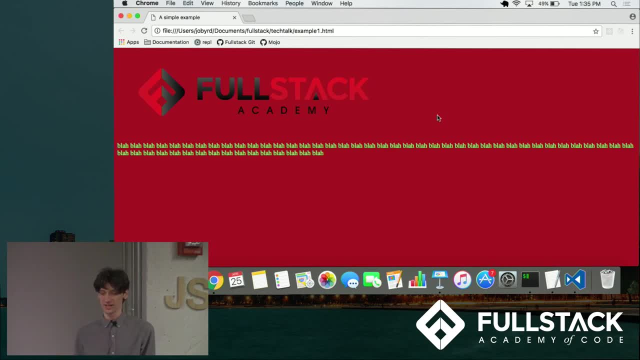 you're probably going to have a lot of trouble reading any of the actual text because it's green on red. This is probably not immediately apparent to most people and it doesn't even affect most people, But it's still there, And you want your website to be able to be accessed by every person.